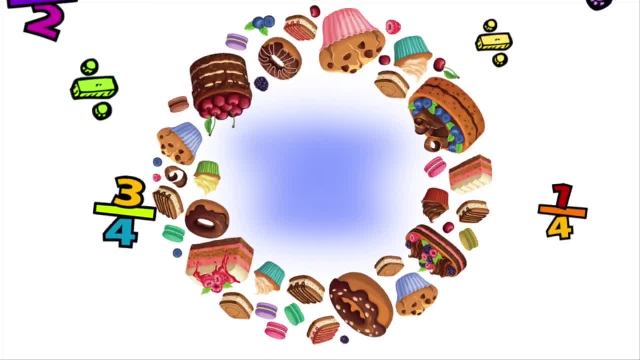 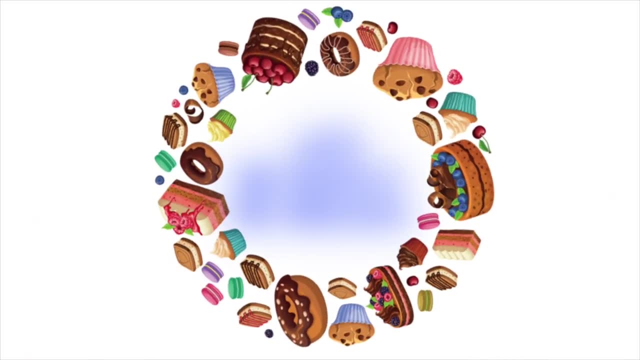 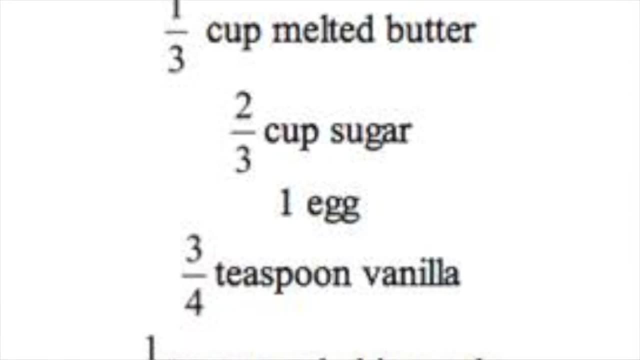 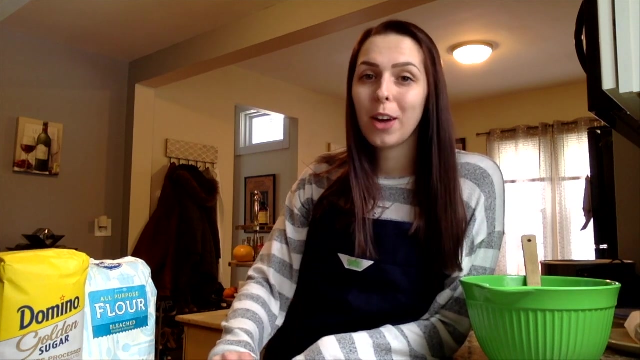 Welcome to Baking with Ms Roeger, and today we're going to be making some banana bread. As you can see, this recipe has a lot of fractions. Now I need to double this recipe so I can make a loaf of banana bread for my grandma, and I'm having trouble doubling these fractions. I'm going to 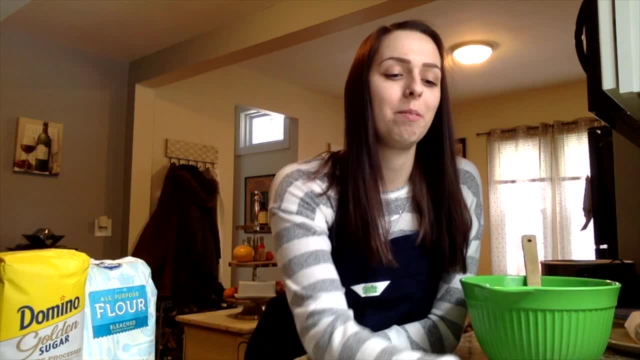 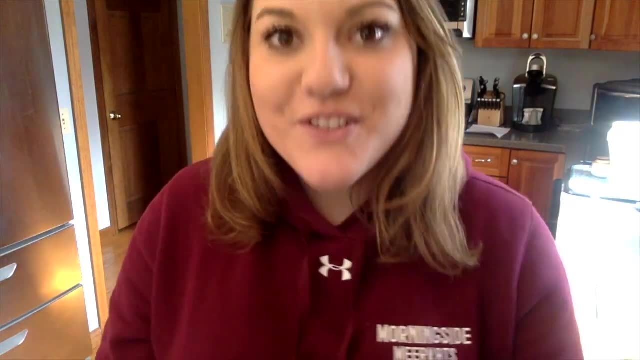 give my friend, Ms Marcella, a call to see if she can help me. Ms Roeger, how are you? I'm doing great. Can you help me with math? Sure, Showing good character at Morningside means helping our. 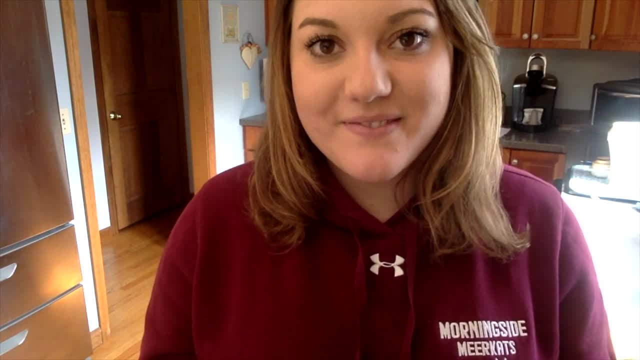 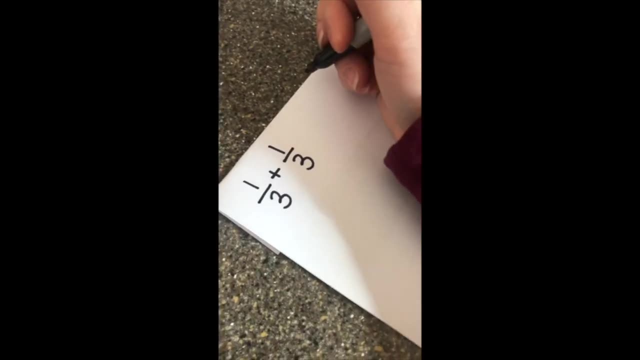 friends, How can I help you? Well, I need to double a recipe with fractions and I do not know how to multiply them. It's simple: You can just use repeated addition. I'll show you. If you want to double the butter, just add one-third plus one-third Since the denominators. 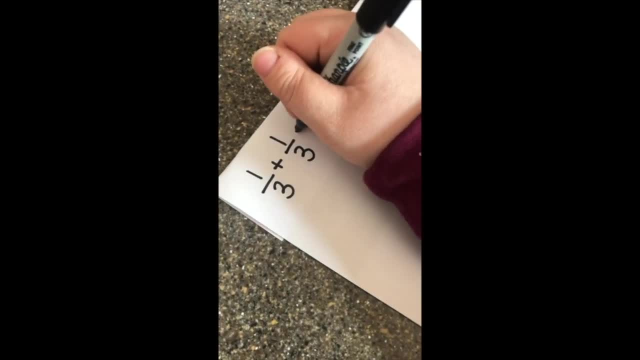 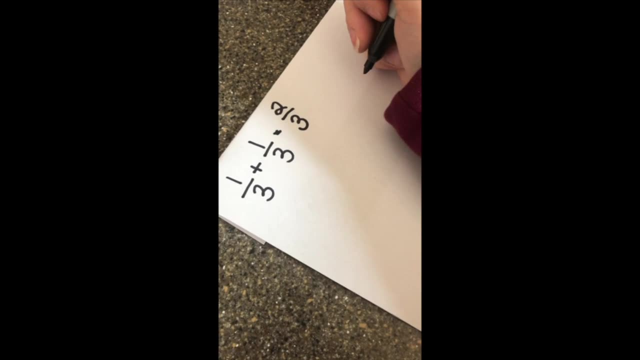 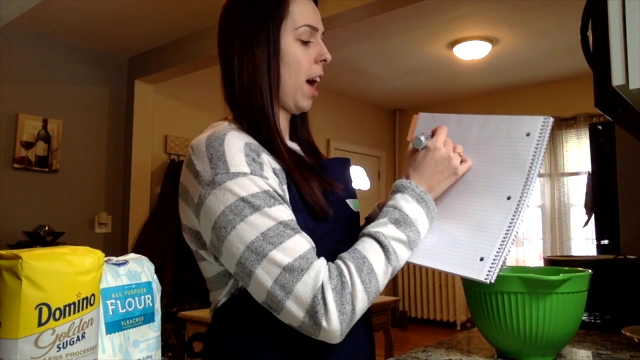 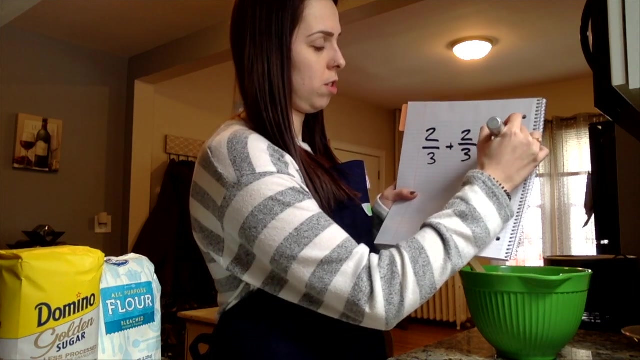 are both the same. we just have to add our numerators: One plus one equals two and our denominator stays the same. So you would need two-thirds cups of butter. That is easy. So if I want to double the sugar, I would do: two-thirds plus two-thirds equals four-thirds. Wait, Ms Marcella. 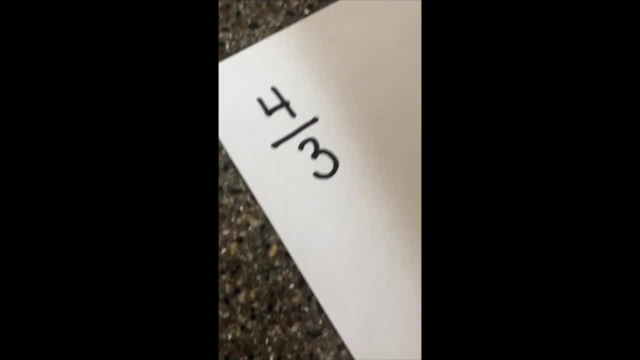 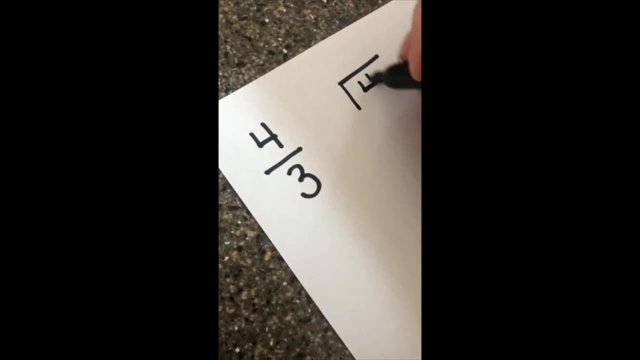 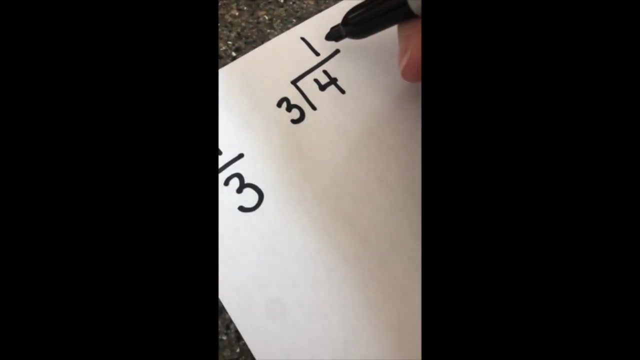 that's an improper fraction. What do I do now That you can change four-thirds into a mixed number? The first is by dividing. Ask yourself, how many times can three go into four? Just once. That's my new whole number. One times three is three, and when I subtract I get one. That's my 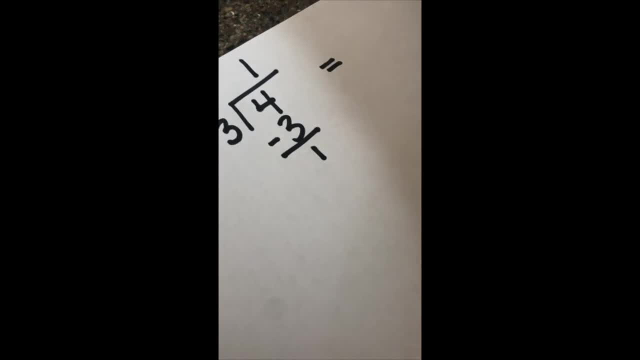 new numerator. My denominator stays the same, So four-thirds as a mixed number is one whole and one-third I can also do a sum of unit fractions. I would add one-third four times, Then I would chunk three-thirds to make one whole and I'm left with one-third.